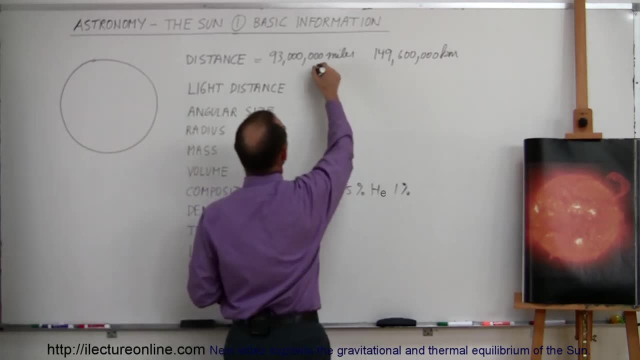 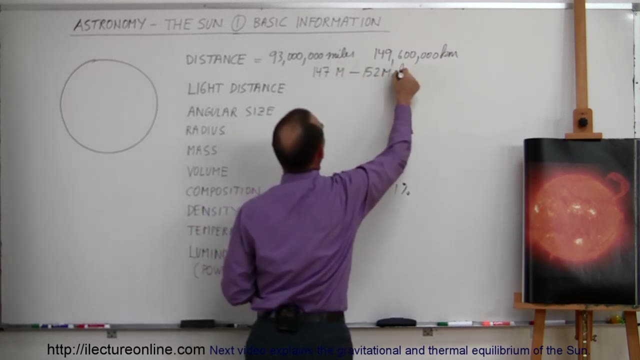 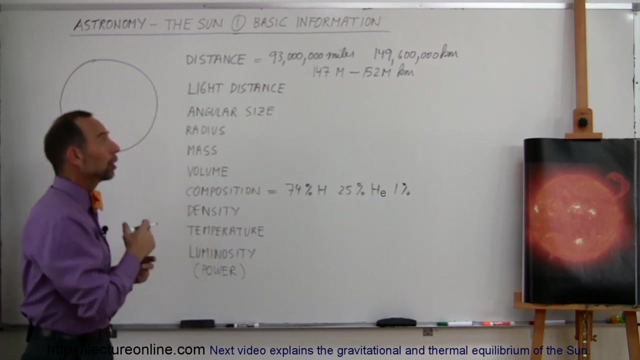 a bit farther away, So typically the earth. the distance between the earth and sun varies from about 147 million to about 150,000 kilometers, So there's about a 3% difference in the distance to the sun from one point of its orbit to the. 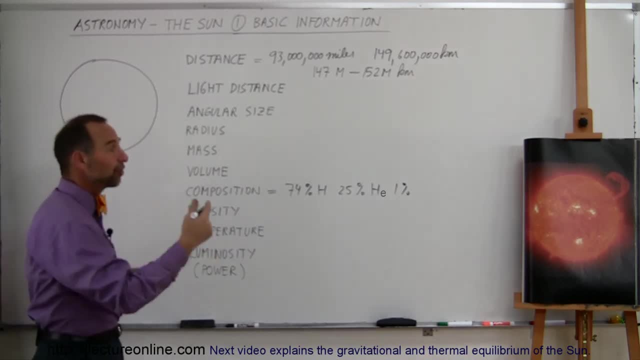 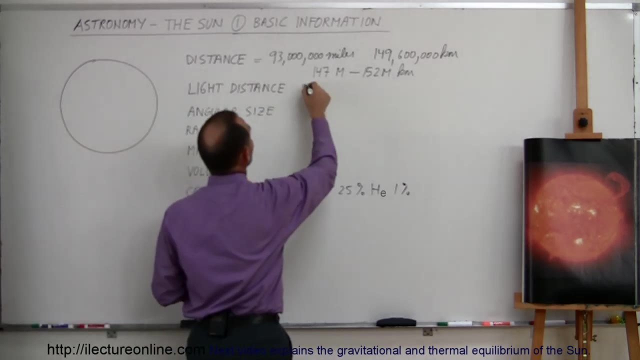 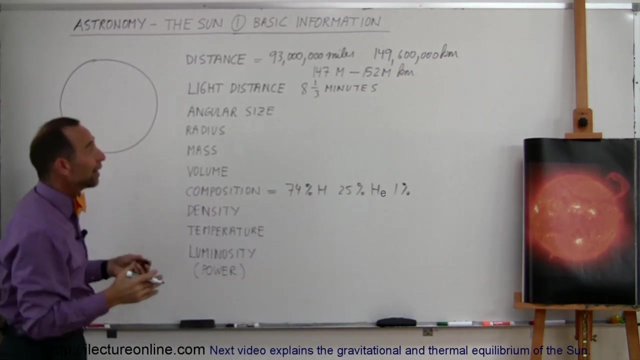 other point of its orbit, Light distance wise. how far is the sun in light units or light travel units? Well, it takes light about eight and a third minutes. So about eight and a third minutes for light to travel from the sun to us. So the distance between the sun and us is about eight. 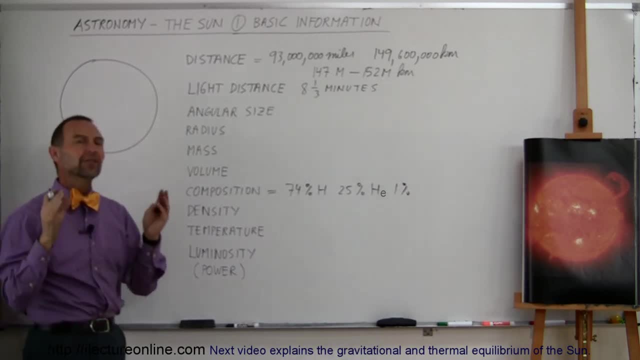 and a third light minutes. Angular size. how big does the sun look? Well, it's about eight and a third light minutes when we look at it in the sky. And so when we look at it from our vantage point- the earth- and we want to measure the what we call the angular size of the sun, it's slightly. 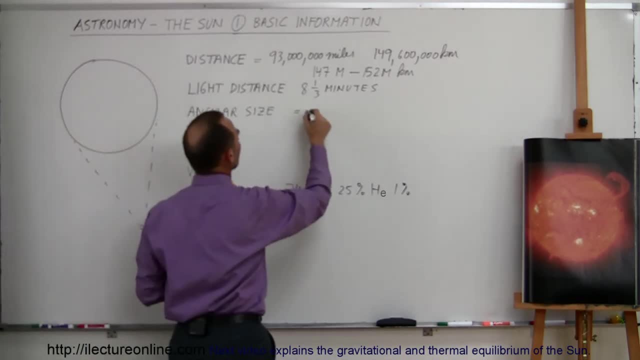 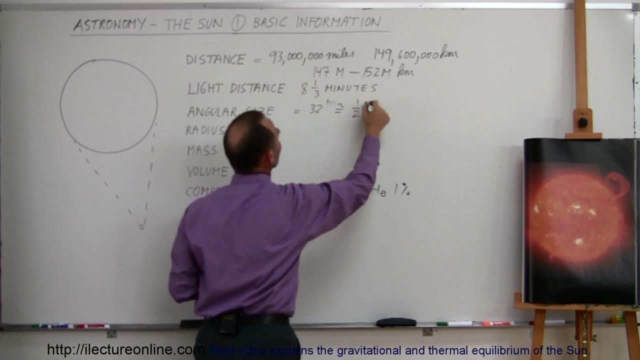 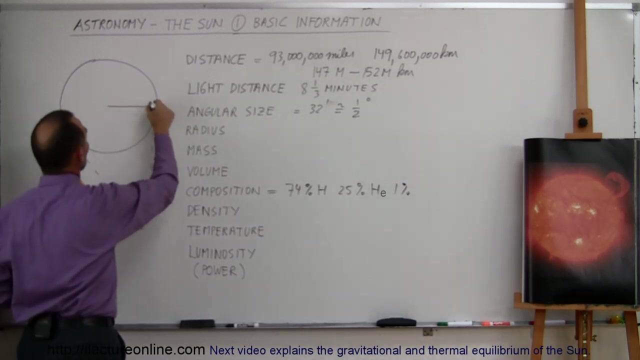 over a half a degree. It's about 32 arc minutes, as we call it. So this is not arc seconds, That would be very tiny arc minutes. So it's roughly about one half of a degree in size. angular size in the sky, Radius wise. how big is the sun in radius? Well, the radius is about 696,000. 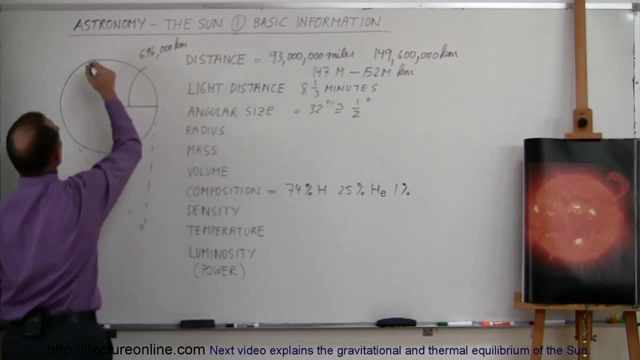 kilometers. That's quite a big, because if you compare that to the earth, the radius of the earth is about 6,378 kilometers, So you can see the vast difference between those two. It turns out the radius of the sun is about 109 times the radius of the earth. Wow, that is quite big. So. 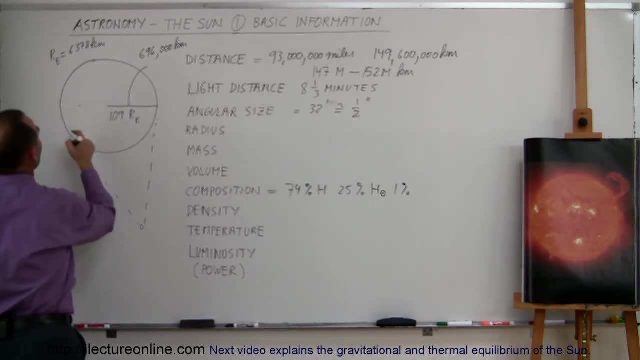 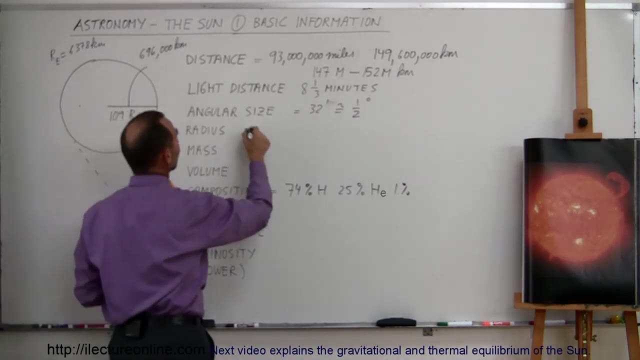 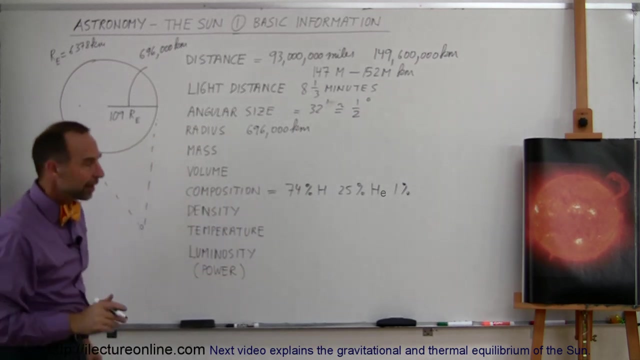 when we were to draw the earth there, it would just be a tiny little spot like that on the sun's surface. The earth is very, very tiny compared to the sun, but the sun is enormously large, of course. So we can say here 696,000 kilometers Mass wise, the density of the sun. 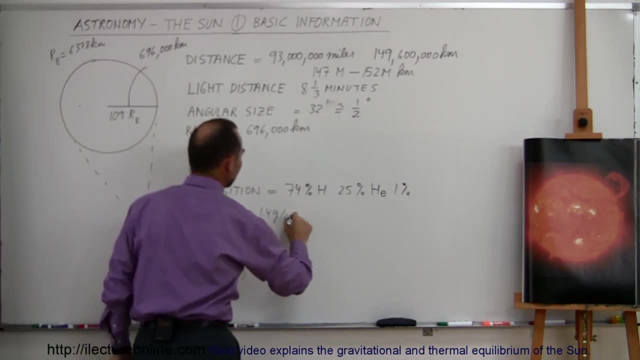 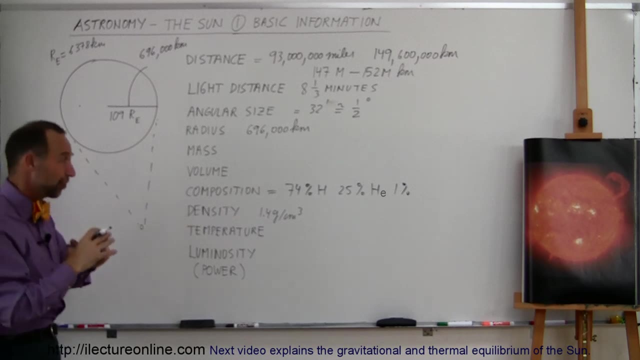 is about 1.4 grams per cubic centimeter. That's the average density, So it's a little bit denser than water on earth, but it turns out at the very center of the sun is much more dense. At the very edges of the sun it's a lot less dense, but on average it's about 1.4 grams per cubic centimeter. 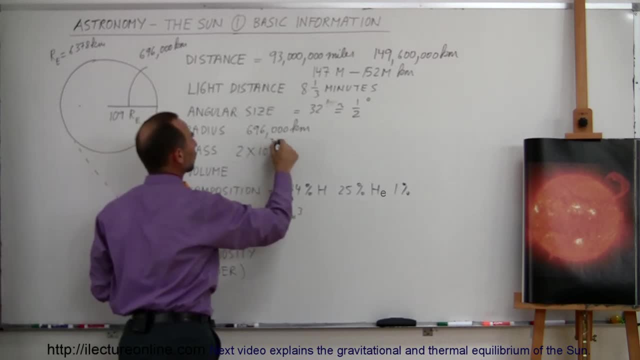 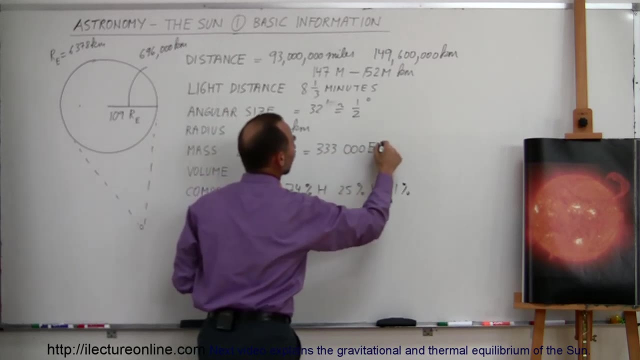 which gives us a mass of about two times 10,000 kilometers. So that's about 1.4 grams per cubic centimeter, which is the mass of about 333,000 earths. I think it's a little bit less. I'm. 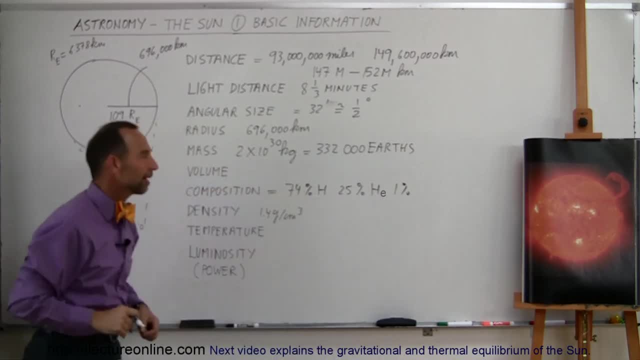 exaggerating. I think it's about 332,000.. Who cares about a thousand earths or not, When it comes to that many, it doesn't make a lot of difference. But in other words, if you were to put the sun, 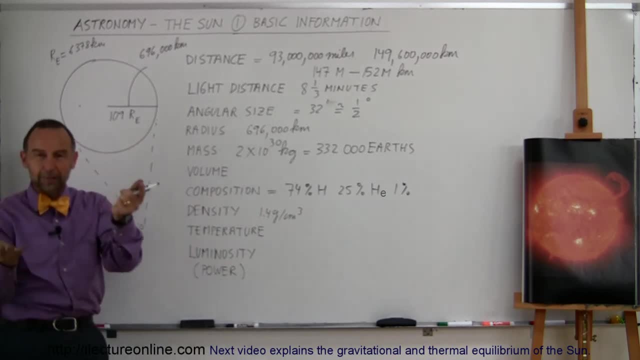 on a scale on one side and you want to put earths on the other side to balance it out, you would need 332 earths to balance out the weight of the sun compared to the weight of the earth or the mass of the sun. 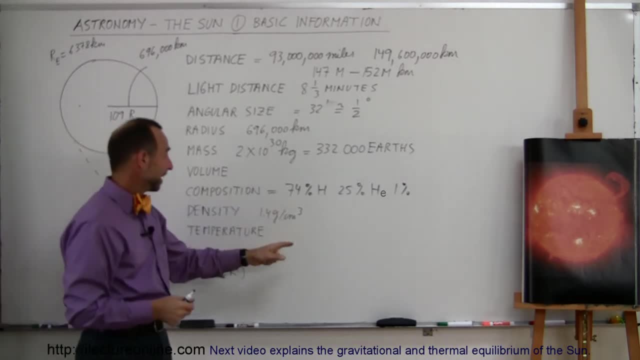 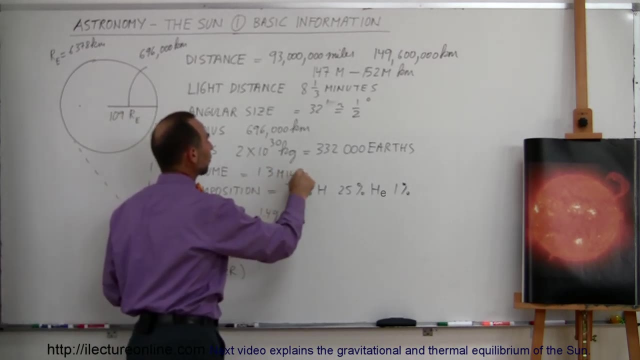 Volume-wise, since the sun is less dense than the earth by quite a factor, you would need about 1.3 million earths to fill up the sun. In other words, if the sun was hollow and you could open it up and start filling it in with earths, put earths in it, you would need 1.3 million earths. 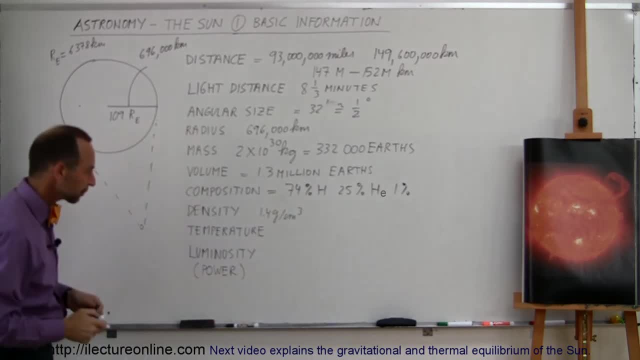 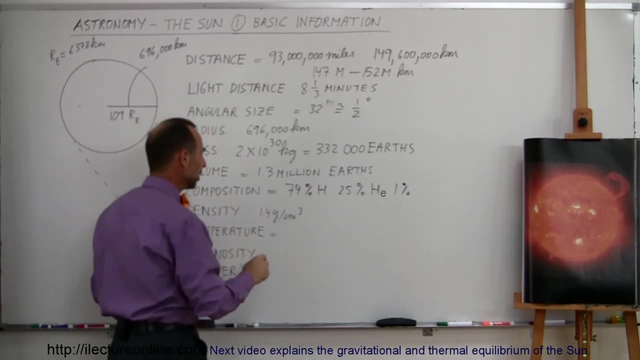 to fill the sun. So the sun is just an enormously large object. Temperature-wise, on the surface the temperature of the sun is about 5.5 degrees Celsius. That's about 5 degrees Celsius, 5,700, 5,800 degrees Kelvin. So I like to use the 5,800 number, and we'll see later why. So it's. 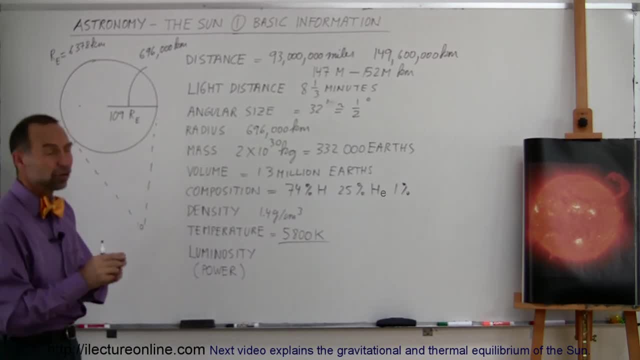 about 5,800 degrees Kelvin on the surface. That is quite hot. There's no substance in the universe that will not be in a gaseous form at the surface of the sun. It's just absolutely too hot. So any substance, any metal, no matter how hard it is, will completely vaporize at a temperature of 5,800. 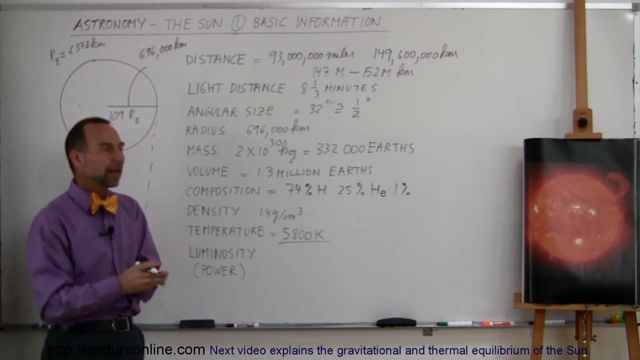 Kelvin Luminosity means how bright is the sun? Now, the sun is a very, very bright sun. It's not a bright star, It's a brighter, it's a bigger star than average, but there's many stars that are. 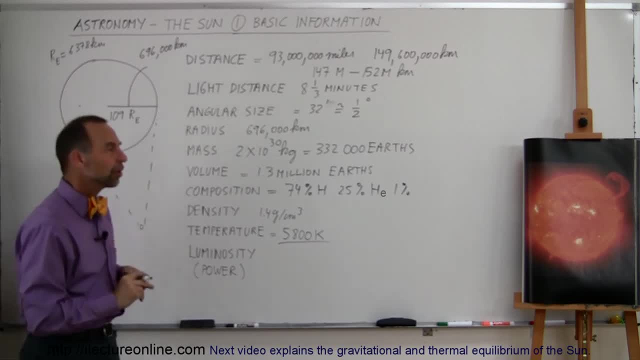 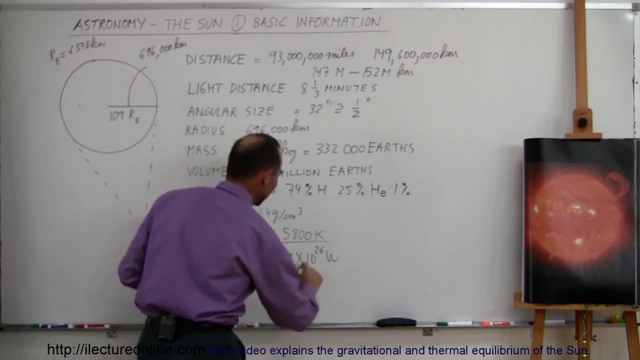 much bigger and much more luminous out there, But for a star the sun does pretty well. The luminosity of the sun is about 3.9 times 10 to the 26 watts. That's the amount of energy that the sun 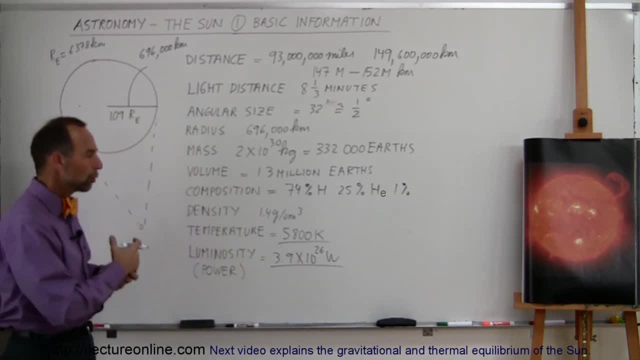 spews out per unit time, The amount of joules per second or the amount of watts. Now you remember, light bulbs are rated in terms of watts. We have 13-watt light bulbs and 26-watt light bulbs. 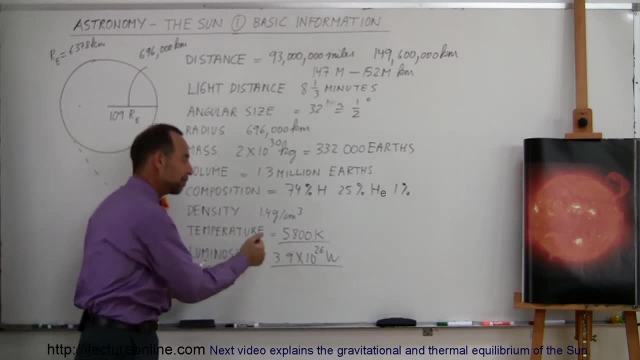 and 50- and 100-watt light bulbs. Well, here's the light bulbs. We have 13-watt light bulbs and light bulb 3.9 times 10 to the 26 watt. How much is that? What enormous amount of energy does the 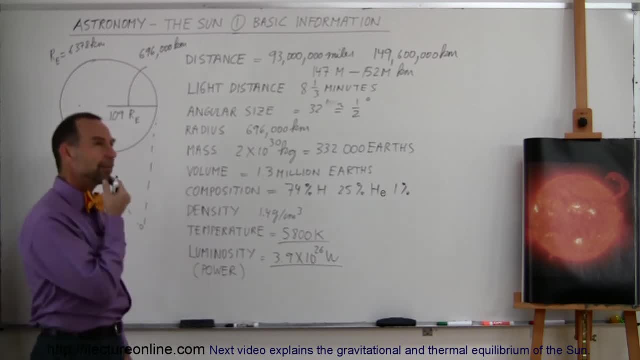 sun provide for us. Well, it's a huge number. So I thought: well, maybe I can figure out how many power plants you would need to generate the same amount of energy. I thought that would be a kind of nice comparison. So I did some calculations and the typical new power plant puts out about a half. 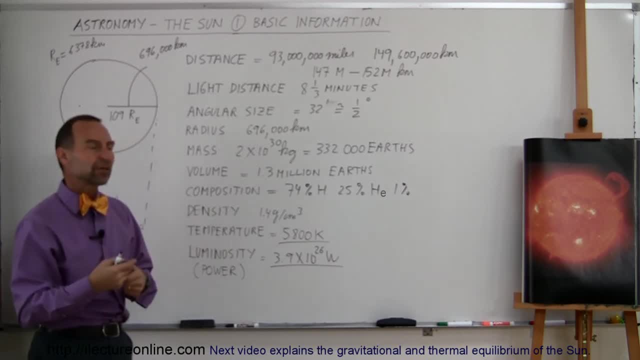 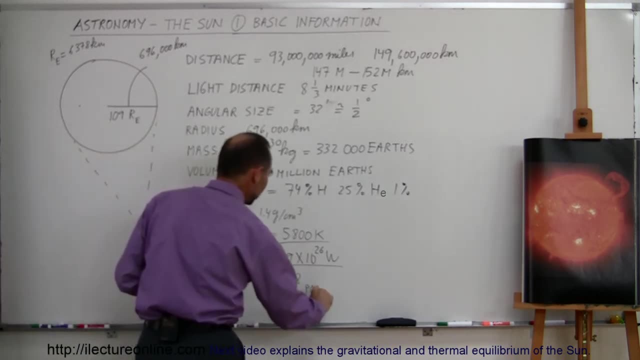 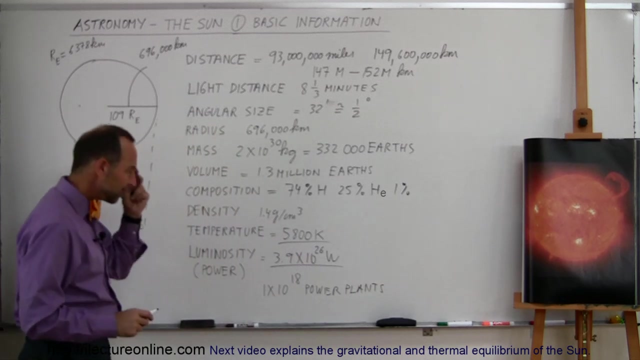 a gig, a gigawatts of power, about 500 million watts of power, And so you would need 1 times 10 to the 18th power plants, A typical new power plant that we build on the earth to provide the same amount of energy as the sun. How big is that number? Well, I believe that number is quintillion. 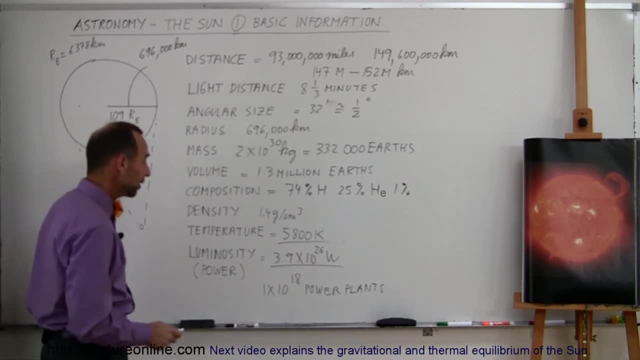 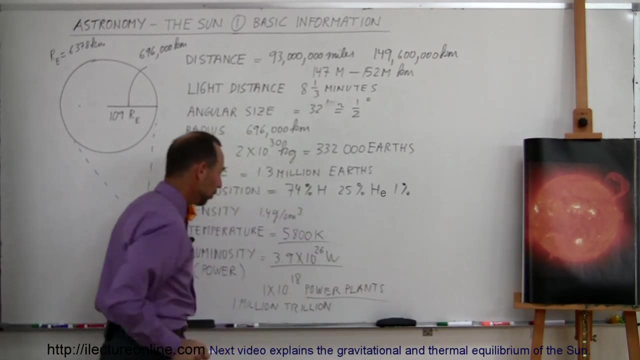 and that doesn't mean a lot to most people. So the way to think of it is it's about 1 million trillion power plants. So if you need to build enough power plants to put out as much energy as the sun would, you would. 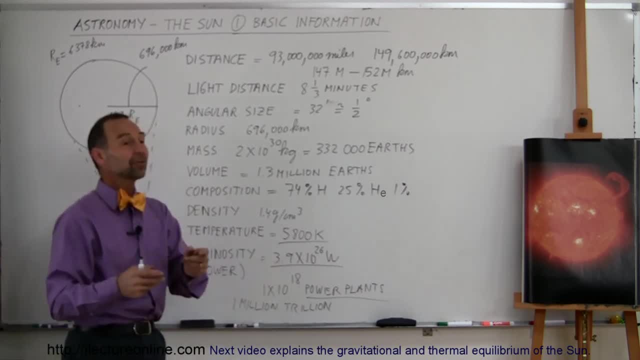 need to build 1 million trillion power plants, not a trillion, not 2 trillion, not a thousand trillion. a million trillion power plants to put out the same amount of energy as the sun. You can imagine you couldn't have enough surface space on the earth to build that many power plants on the 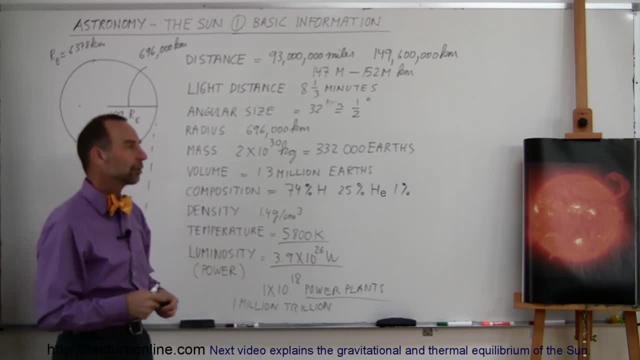 earth. The earth would be way too small. It's just an absolute amount of power that the sun provides. But it gives you kind of an appreciation about what that thing is, What that thing is up there that keeps us alive. The sun is basically the source of all life on earth. 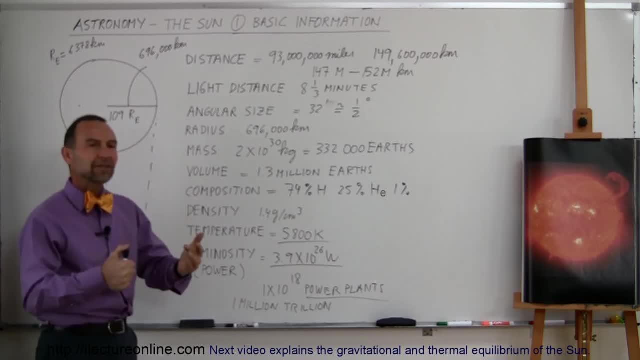 It provides us with the warmth, the energy, the energy that the plants need in order to grow, so they can use their chlorophyll to turn carbon dioxide into oxygen, so we can breathe, and it can provide us with food for us to eat and food for all the animal life that's out there. Just the sun is just absolutely the one item up. 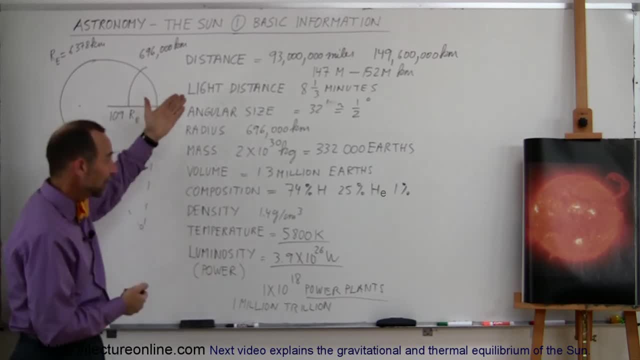 there that keeps the entire earth going and keeps us alive, And these are the specifics of that thing. up there, And as we go on through the next so many videos, we'll start showing you what an amazing thing that is. We'll start learning more about the sun and what the sun is and how the sun 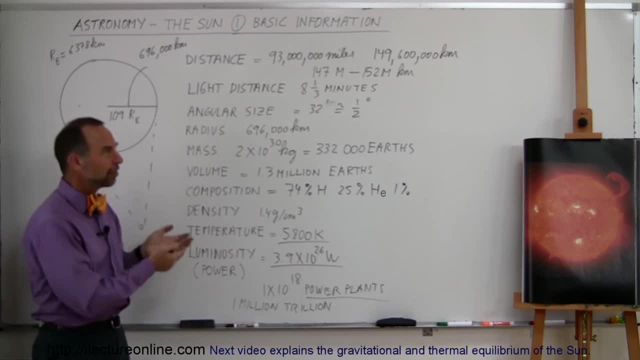 produces energy and so forth, what kind of cycles it goes through. But anyway, this is a nice little start. That's our sun up there, 93 million miles away, And stay tuned if you're interested in hearing more about the sun.